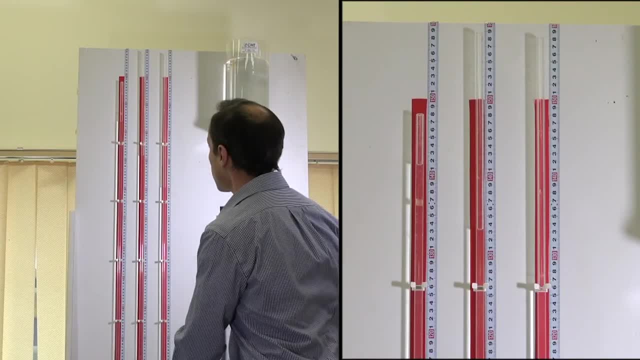 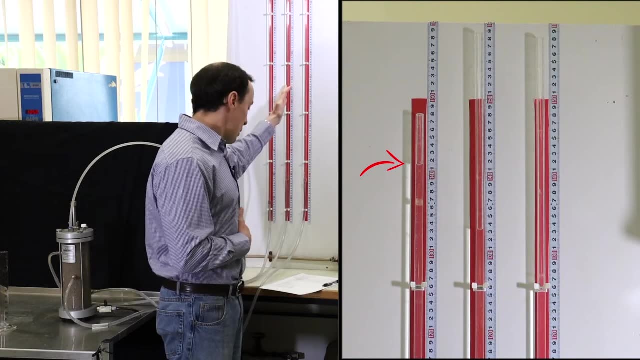 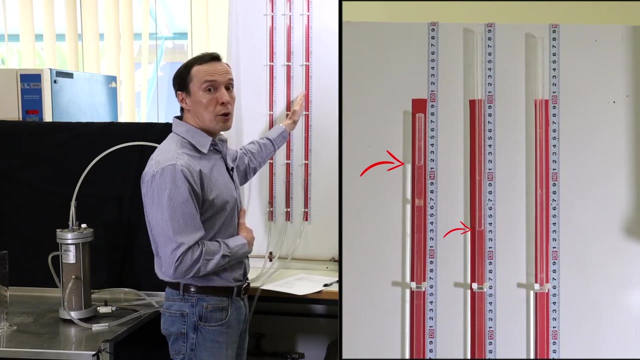 The one on the left hand side, which is connected to the top part of the sample, would give us numbers of 1,411 millimeters. The one in the middle will give number of 1,328 millimeters. The one on the right hand side actually has a number of 1,252 millimeters. 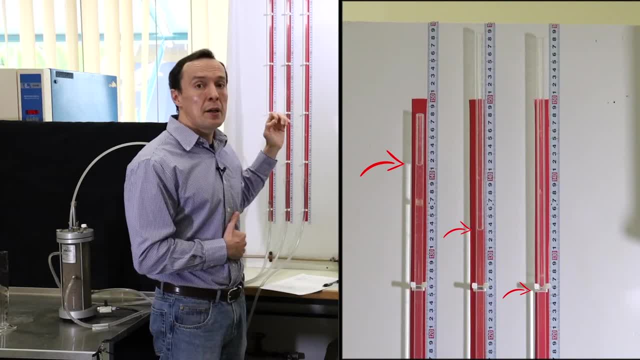 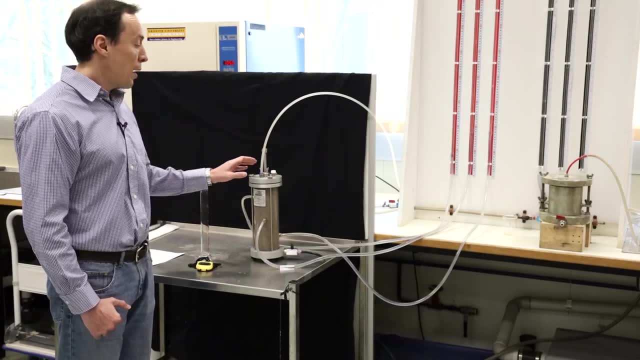 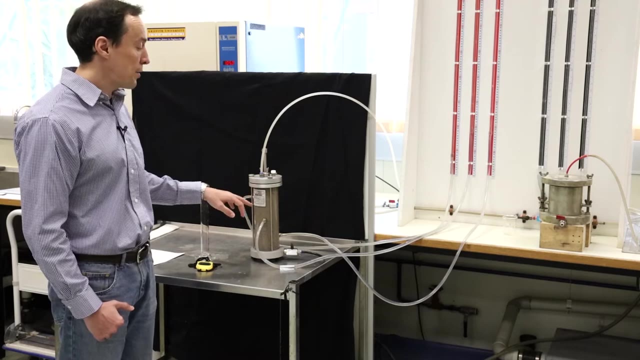 So these are water levels, water heads that now are active in the soil sample during the test. When water flows through the sample and it's on the constant flow, we'll see that when we measure of water levels on these three manometers they will be the same. They will be. 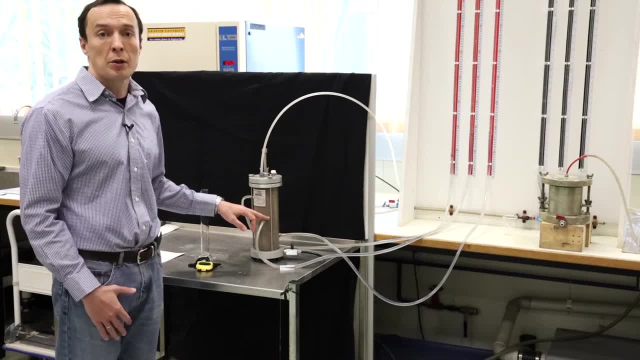 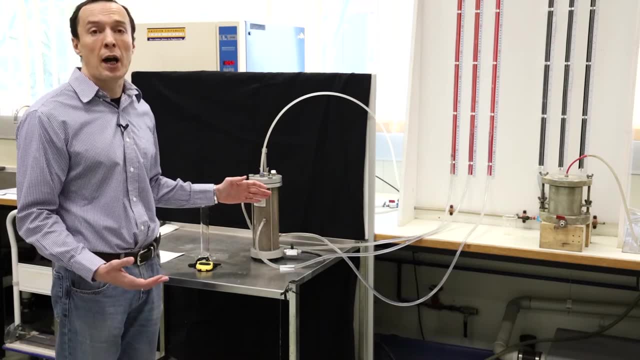 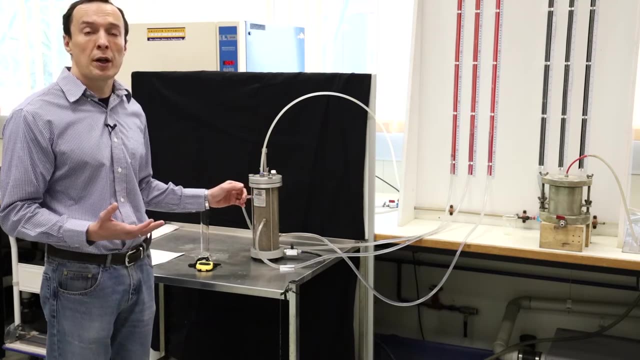 constant. That's why this test is called constant head r test. What we will do now is: I would like to know how much water comes out of the soil over time, so that we can calculate the velocity of water flow. Once we know the velocity of water flow, we can calculate the coefficient of 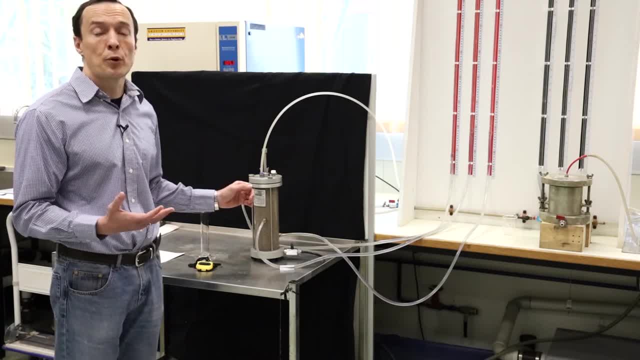 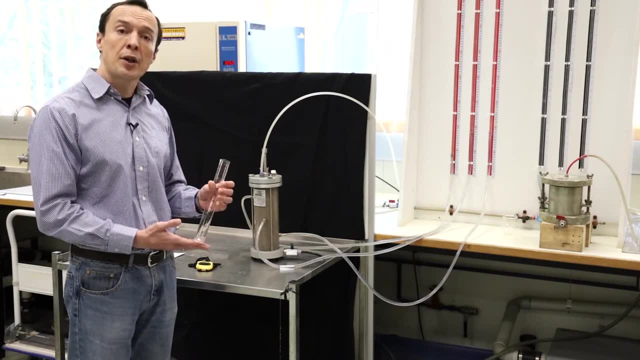 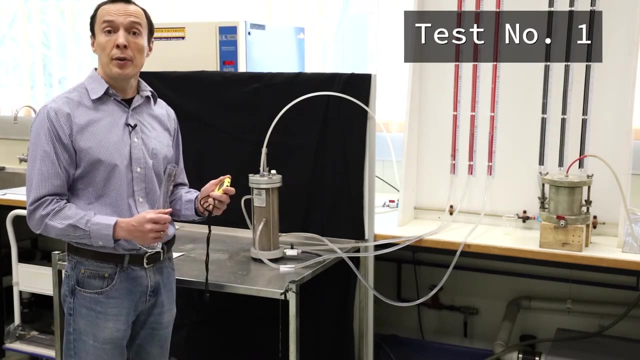 permeability, which is very important property of soil that we would like to get from this test. To do this test, we will use this water container that can measure the amount of water and we will use timer. The test is pretty simple: We would like to know how much water flows in this container over a certain period. 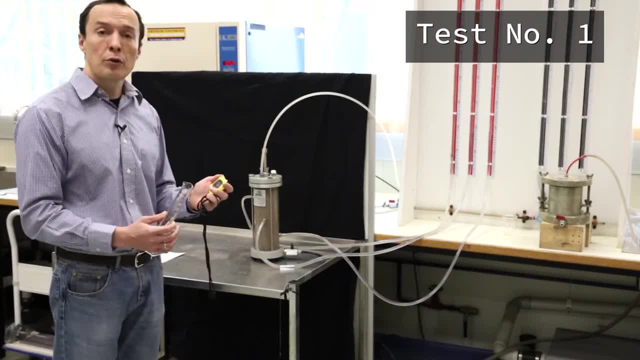 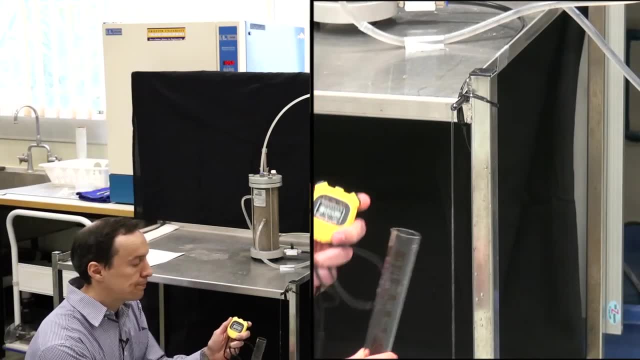 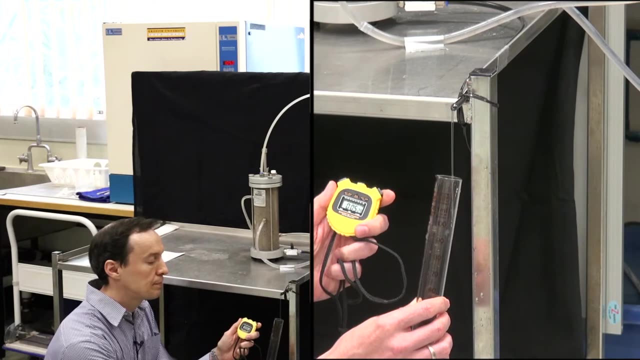 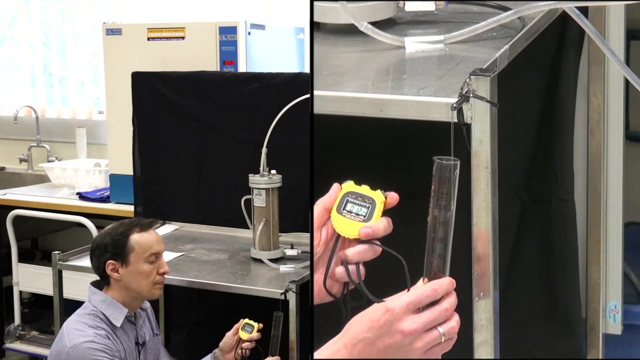 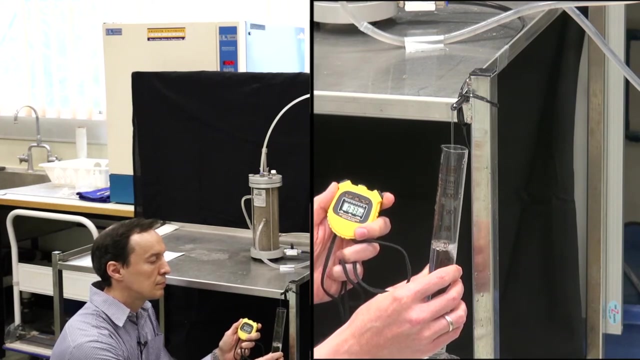 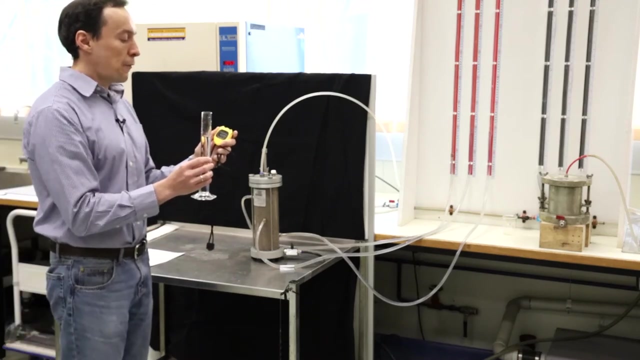 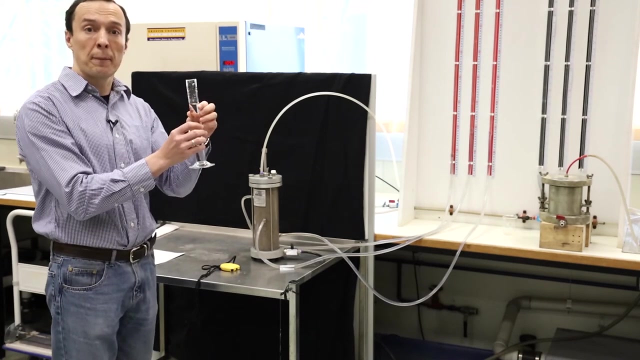 of time, and this is what I'm going to do right now. I'm going to start the timer and collect water at the same time. I'm going to start the timer and collect water at the same time. It takes 43 seconds to collect 92 milliliters of water. We should repeat.